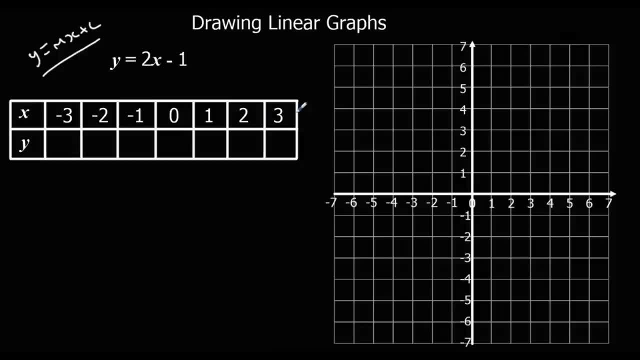 do is we've got to fill out the table of values which will allow us to plot the coordinates on the graph. It's actually easier to start at the right over here, because we started with positive numbers and then we can usually see the pattern that forms. So what we've 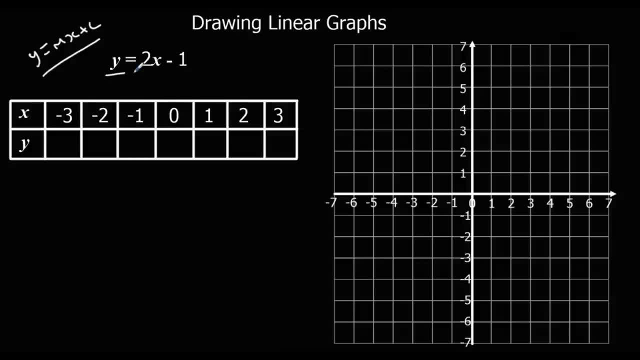 got to do is we've got to substitute the x values into the equation to find the y value. So it's 2 times whatever the x value is. take away 1.. So the y value is 2 times this number. take away 1.. 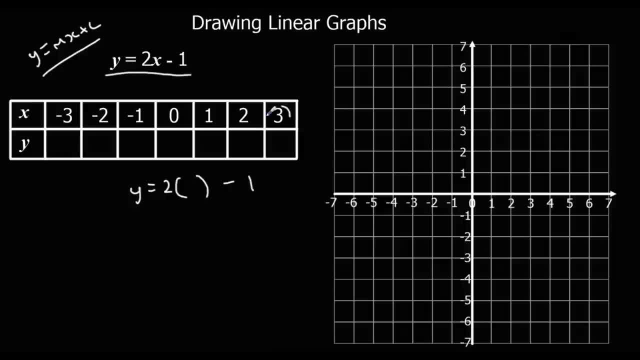 So for the first one we've got 2 times 3, take away 1.. So 6, take away 1,, which is 5.. 2 times 2 is 4, take away 1, 3.. 2 times 1, take away 1, is 1.. 2 times nothing: 0, minus. 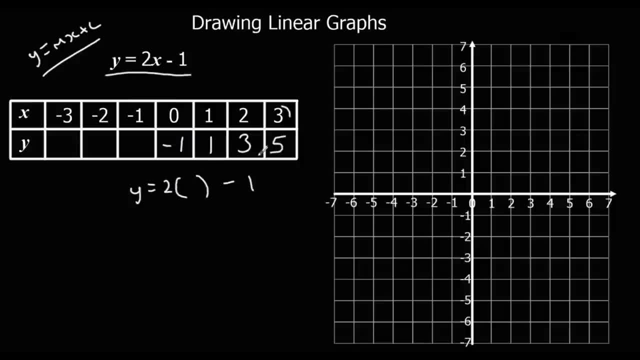 1, is minus 1.. You can see the pattern emerging. already It's going up in twos. So we could carry on with the pattern going backwards. You'll be able to notice if you've made a mistake, because the line won't be straight. 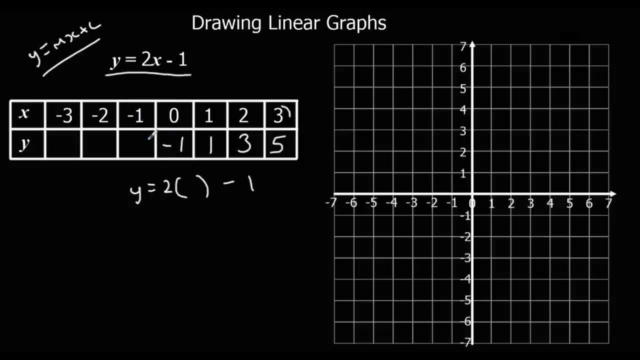 So let's just keep going with this. So 2 times minus 1, minus 2.. Minus 1 is minus 3.. 2 minus 2 is minus 4.. Minus another one is minus 5.. And 2 minus 3 is a minus 6.. Minus another: 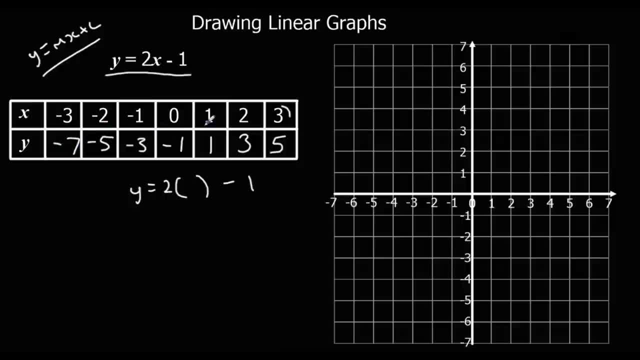 one minus 7.. And then we just these turn into coordinates. So this is a set of coordinates here. So this one turns into 3, 5.. We can plot that in the graph. This one turns into 2, 3.. We can plot that in the graph. 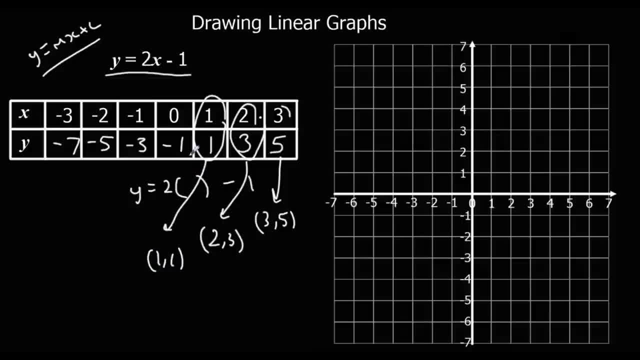 This is 1, 1.. 1, 1. 0, minus 1.. So x first, then y remember, And we can just plot these onto the graph. So 3, 5. 3, 5. 2, 3.. 1, 1. 0, minus 1.. 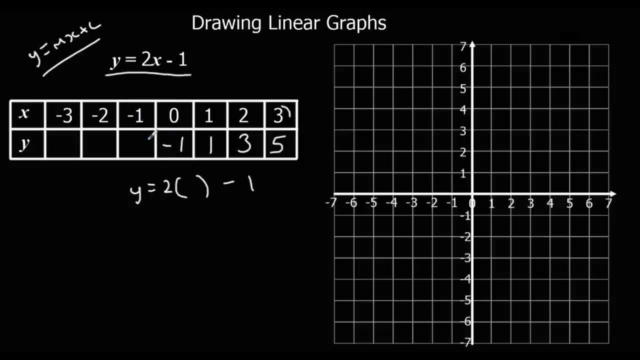 So let's just keep going with this. So 2 times minus 1, minus 2.. Minus 1 is minus 3.. 2 minus 2 is minus 4.. Minus another one is minus 5.. And 2 minus 3 is a minus 6.. Minus another: 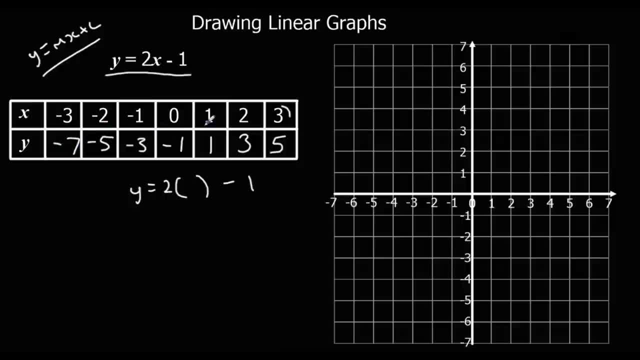 one minus 7.. And then we just these turn into coordinates. So this is a set of coordinates here. So this one turns into 3, 5.. We can plot that in the graph. This one turns into 2, 3.. We can plot that in the graph. 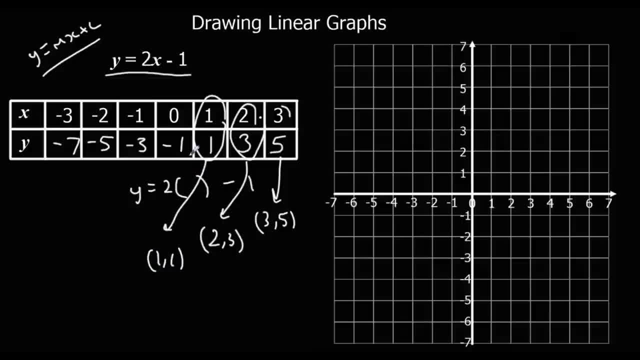 This is 1, 1.. 1, 1. 0, minus 1.. So x first, then y remember, And we can just plot these onto the graph. So 3, 5. 3, 5. 2, 3.. 1, 1. 0, minus 1.. 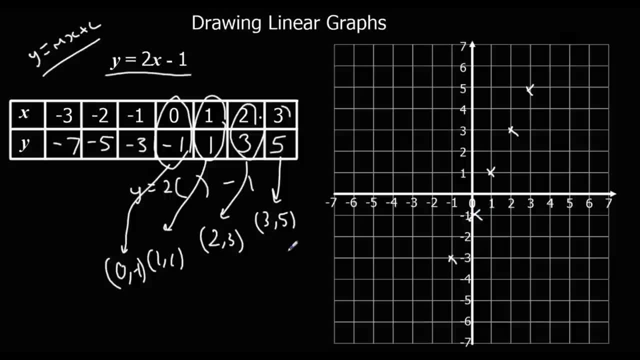 We've got minus 1, minus 3.. Minus 2, minus 5.. And minus 3, minus 7.. So we've got a straight line that's formed up there, which is what we wanted, And then we can just draw a straight. 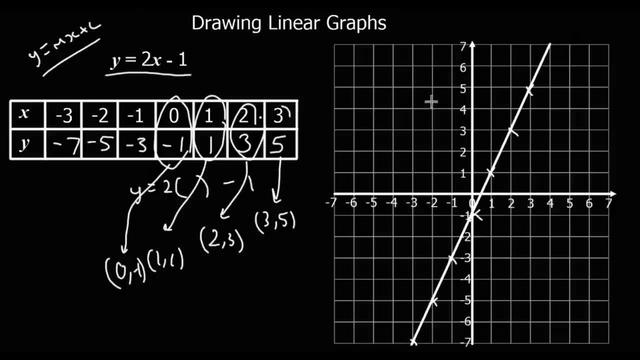 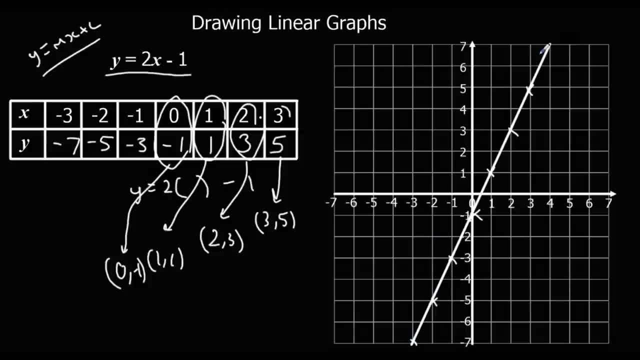 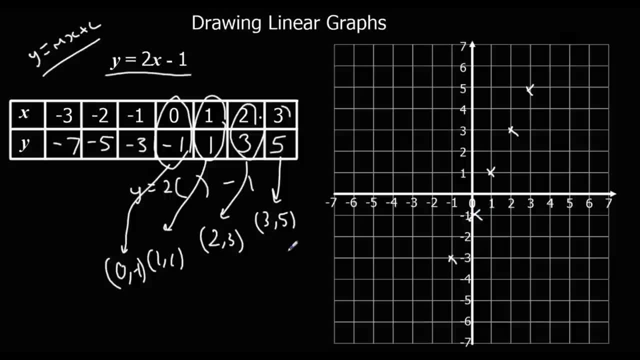 We've got minus 1, minus 3.. Minus 2, minus 5.. And minus 3, minus 7.. So we've got a straight line that's formed up there, which is what we wanted, And then we can just draw a straight. 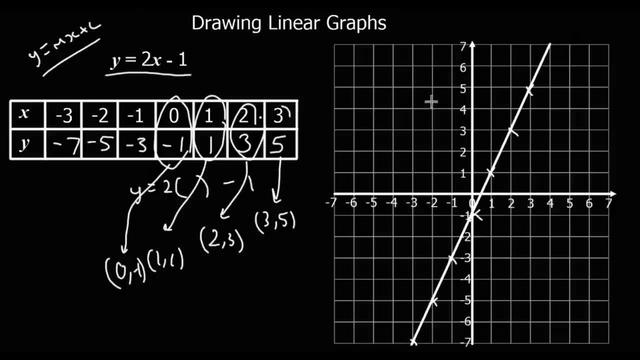 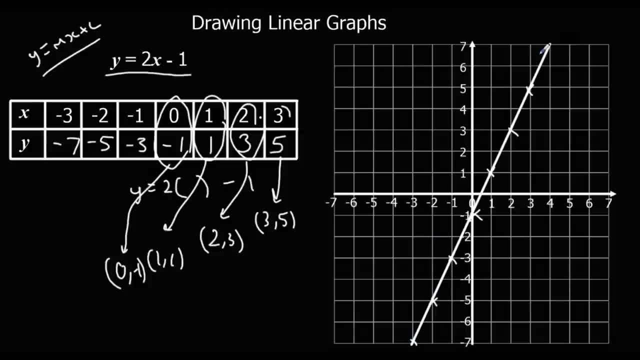 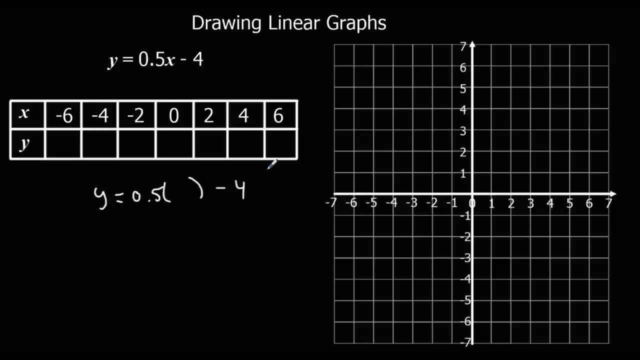 half times. whatever our number is, take away 4.. So we can just substitute our numbers in. So I'm going to start from the right again, because it's easier to start with positive numbers. So half of 6 is 3.. 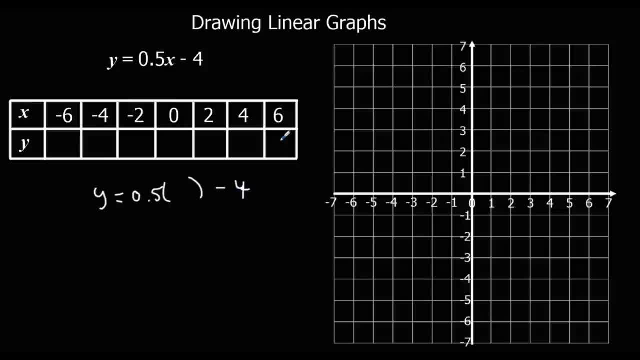 3. take away 4 is minus 1.. Half of 4 is 2.. Take away 4 minus 2.. Half of 2 is 1.. Take away 4 minus 3.. Half of nothing is nothing, And we can see the pattern here: It's going down. 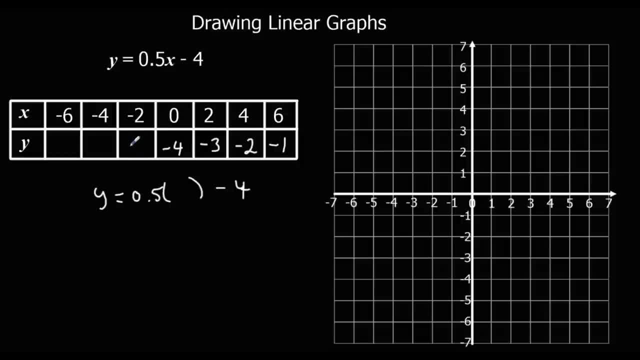 by 1 each time. So we can carry on with the pattern. Or we could have carried on substituting numbers in. So let's draw these coordinates on now. So this becomes 6 minus 1.. This becomes 4 minus 2.. So let's plot these on the graph. 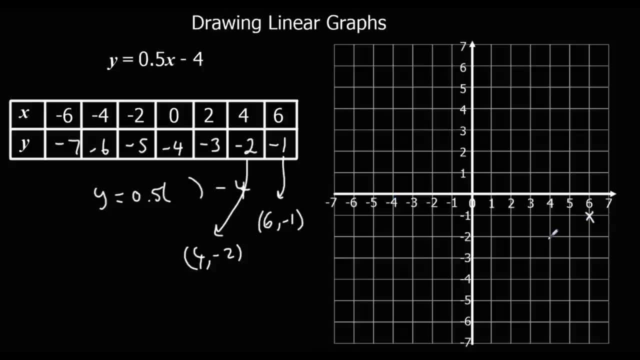 So 6 minus 1.. 4 minus 2.. 2 minus 3. 0 minus 4. Minus 2 minus Minus 5. Minus 4 minus 6. And minus 6 minus 7.. 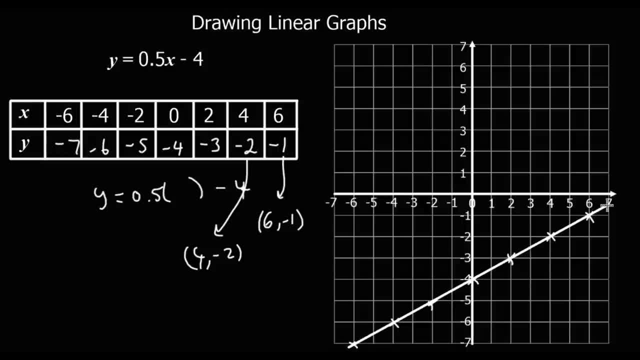 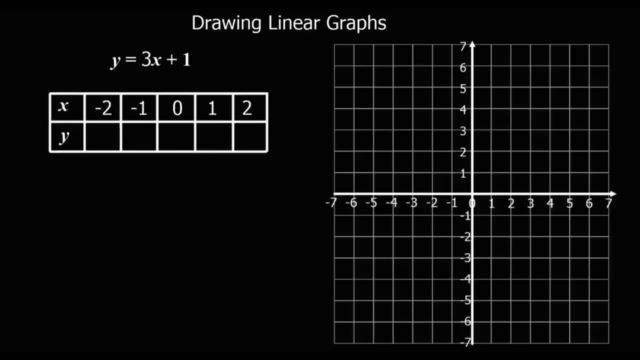 And that's to draw another straight line. So through all the points And it's formed another straight line, so we know we've done it right. Okay, see if you can do this one. So try and fill out the table and then figure out what. 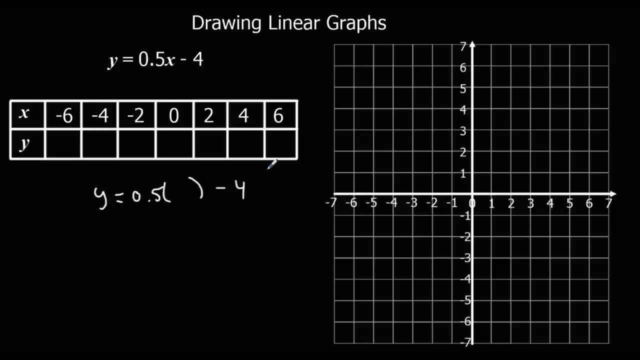 half times. whatever our number is, take away 4.. So we can just substitute our numbers in. So I'm going to start from the right again, because it's easier to start with positive numbers. So half of 6 is 3.. 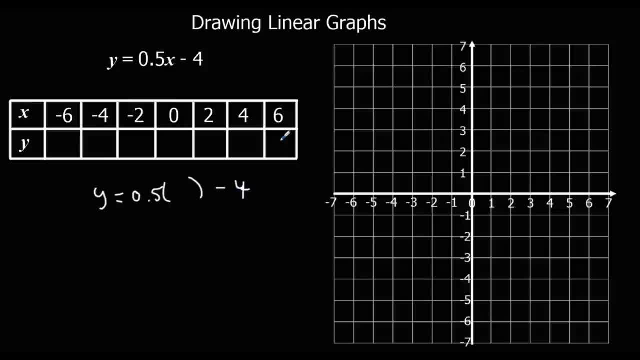 3. take away 4 is minus 1.. Half of 4 is 2.. Take away 4 minus 2.. Half of 2 is 1.. Take away 4 minus 3.. Half of nothing is nothing, And we can see the pattern here: It's going down. 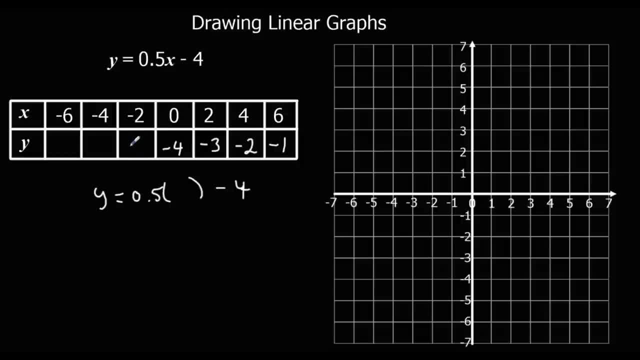 by 1 each time. So we can carry on with the pattern. Or we could have carried on substituting numbers in. So let's draw these coordinates on now. So this becomes 6 minus 1.. This becomes 4 minus 2.. So let's plot these on the graph. 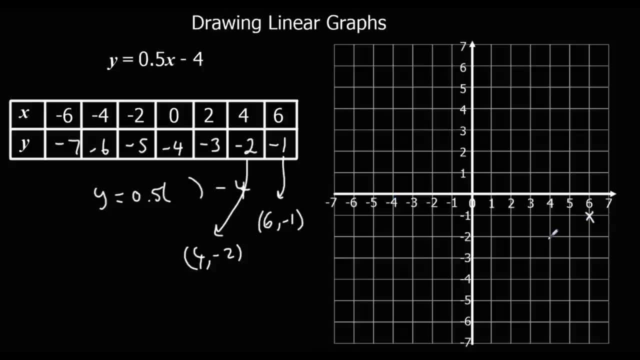 So 6 minus 1.. 4 minus 2.. 2 minus 3. 0 minus 4. Minus 2 minus Minus 5. Minus 4 minus 6. And minus 6 minus 7.. 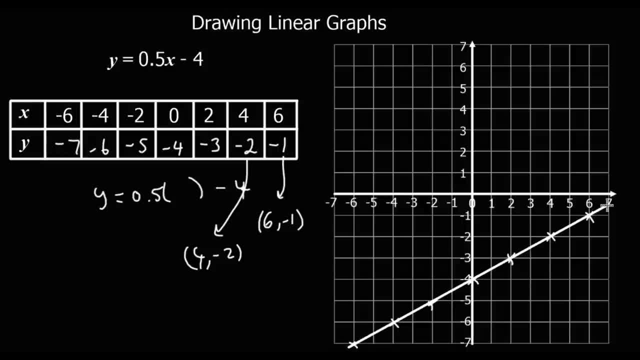 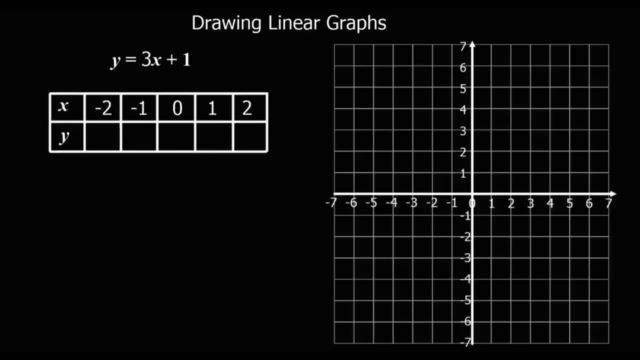 And that's to draw another straight line. So through all the points And it's formed another straight line, so we know we've done it right. Okay, see if you can do this one. So try and fill out the table and then figure out what. 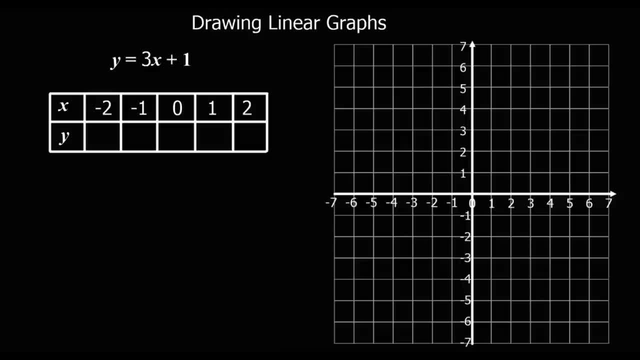 the coordinates are and plot them on the graph. So what we have to do to find the y-values is 3 times our number plus 1.. So 3 times the x plus 1.. So 3 2's plus 1 is 7.. 3, 1 plus 1 is 4.. And we should have got a pattern. 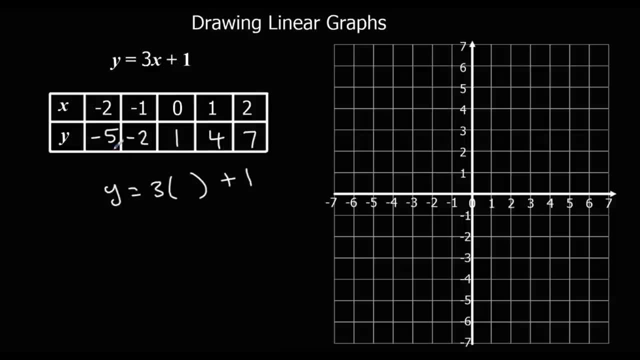 going up in 3's each time. In 3's each time, Then plot in the coordinates, so 2, 7.. 1, 4.. 5, 6. 20. traveled, And what's our number here? 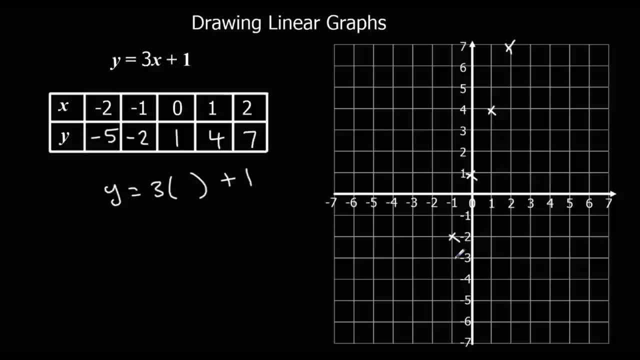 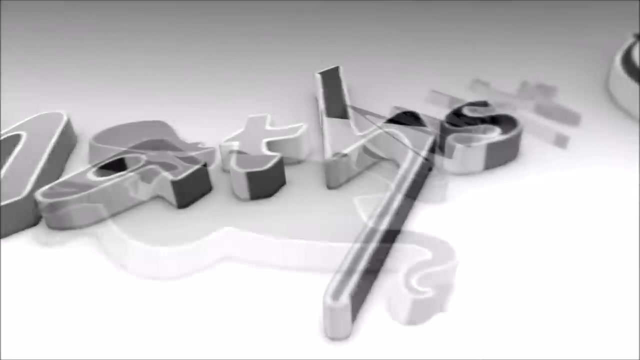 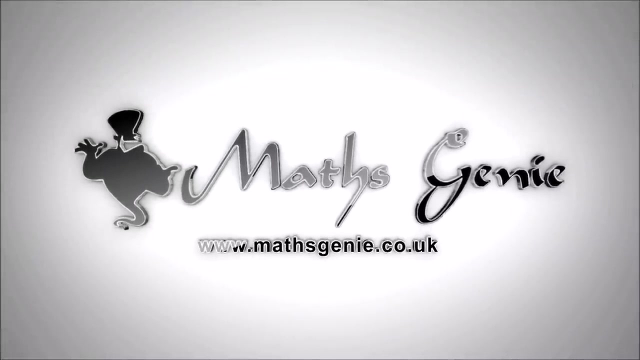 0, 1, minus 1, minus 2, and minus 2, minus 5.. And we draw a straight line that goes through each of the points. It should look something like that. Thank you.